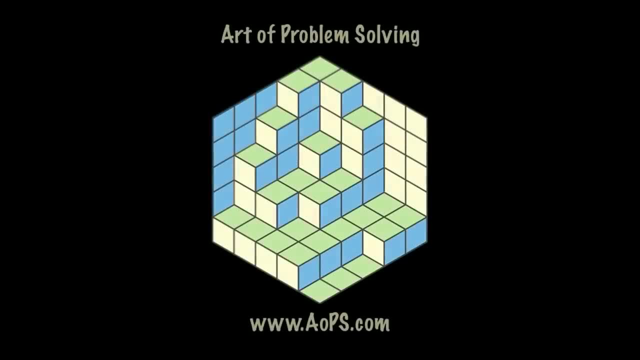 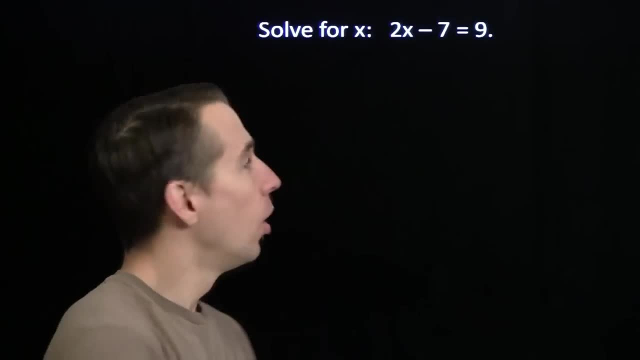 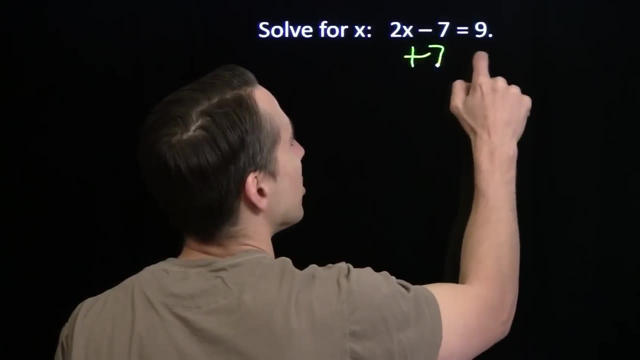 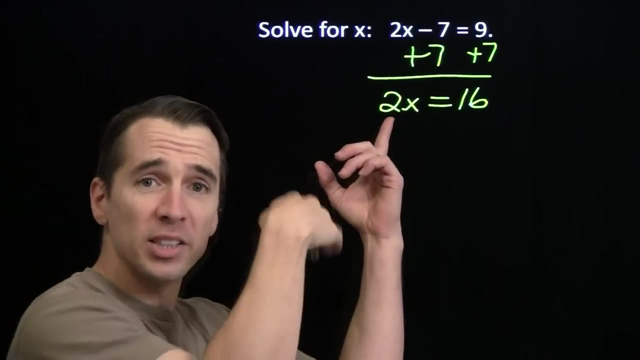 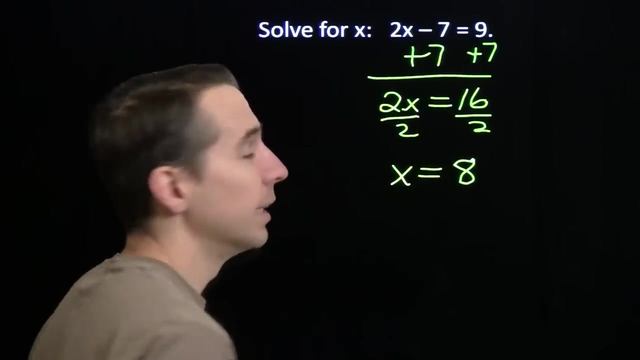 We know how to handle this. We isolate the variable. We start off by getting the 2x all by itself by adding 7 to both sides. That gives us 2x equals 16.. Then we get the x by itself by dividing both sides by 2, and that leaves us x equals 8.. Now, if you watched those last, 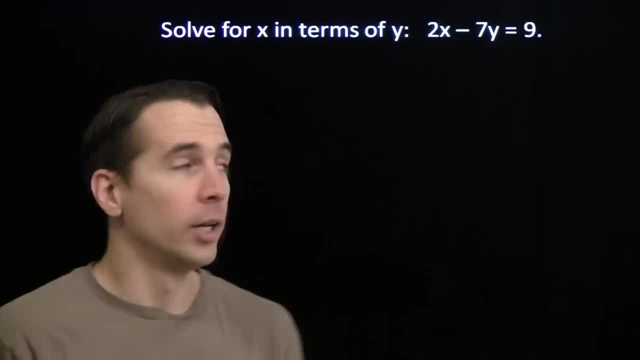 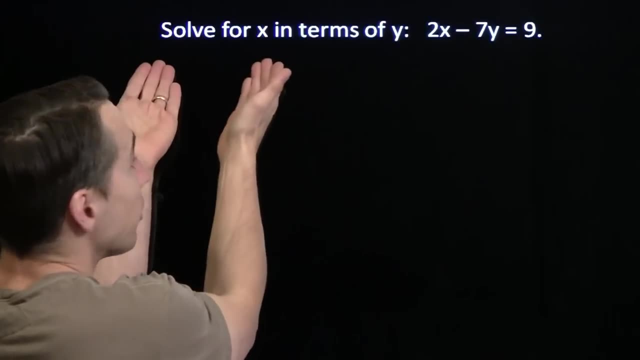 few lessons. you know what we're going to do now. That's right: More variables. And you also know what I'm going to say. There's nothing new here. The name of the game here is solving for x, Just like it was here: solving for x, Only here our final result is going. 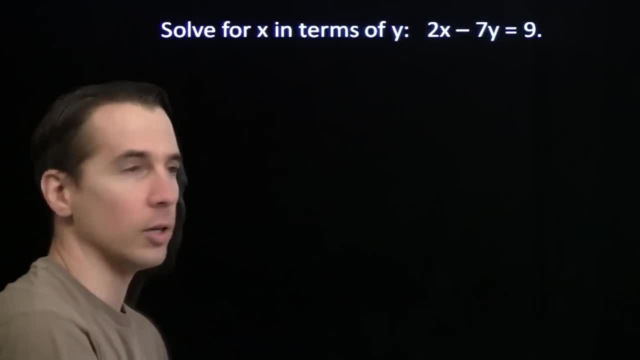 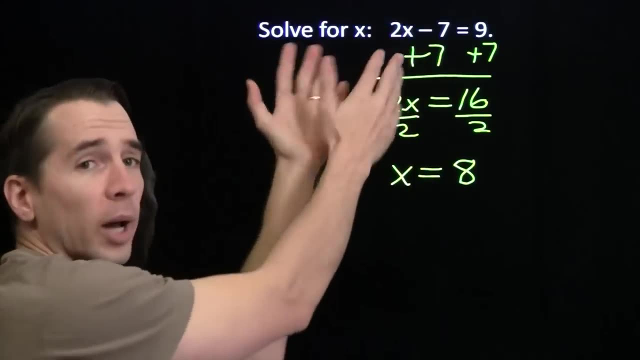 to have some y's on the other side. We're going to have x equals and we're going to have some y's over there, Instead of just having a number Now here, our first step was to isolate the 2x Isolate. 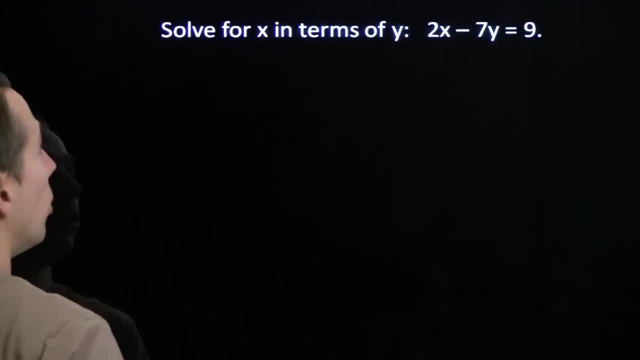 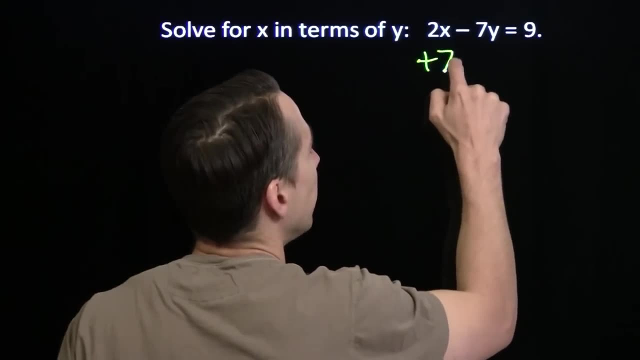 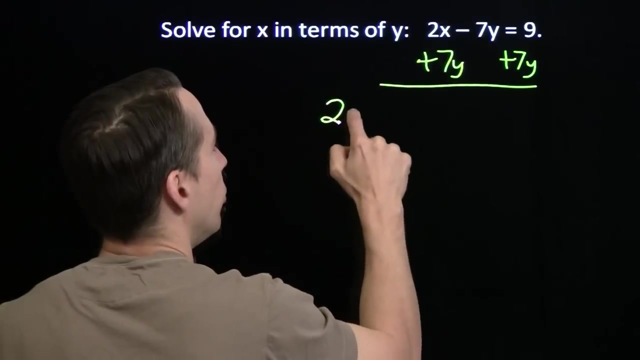 the part of the equation that has x. We do the same thing here. Again, there's nothing new here. You already know how to do this. We'll start off by adding 7y to both sides, And that gives us the 7y's cancel, and over on the left we have 2x And over on the right 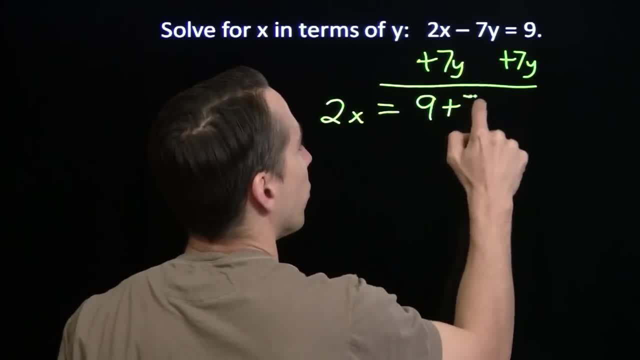 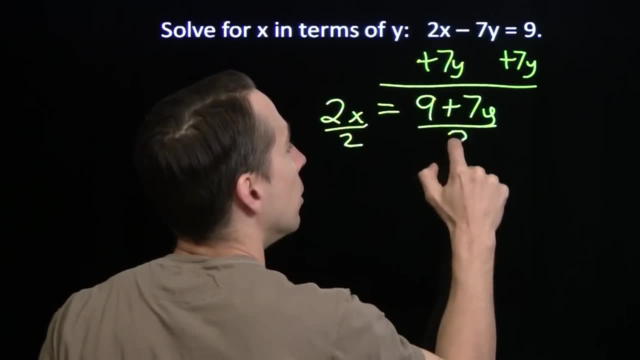 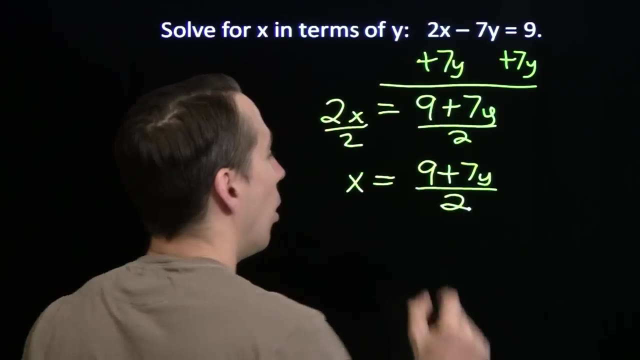 side we have 9 plus 7y, And then we need to get the x all by itself. We divide both sides by 2. And we have x equals 9 plus 7y. All of that divided by 2. And we've solved for x in terms of y And this gives: 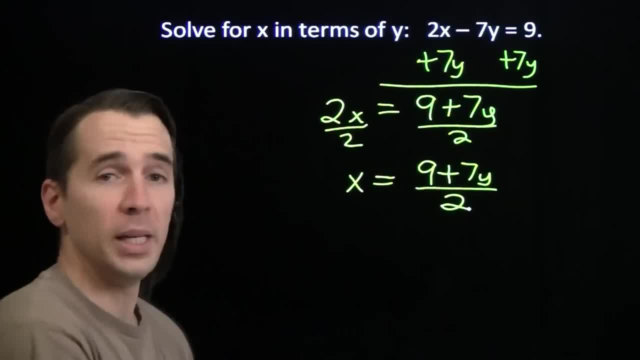 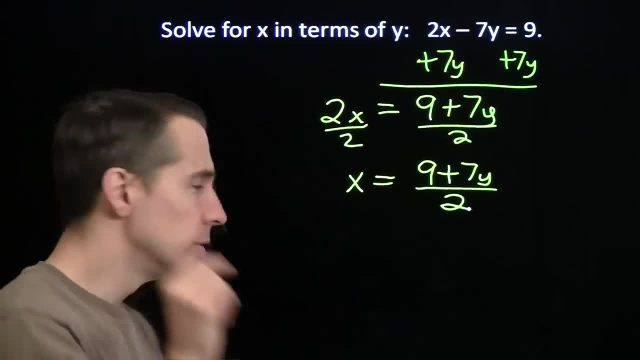 us a formula. So whenever we figure out what y is or decide what we want y to be, we just throw it in here and we'll get the corresponding x, such that those x and y satisfy this equation. Let's give it a try. 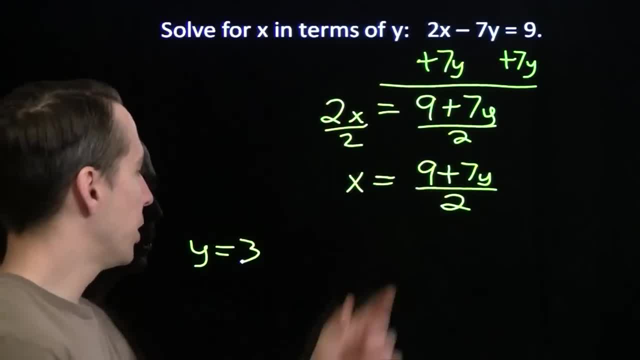 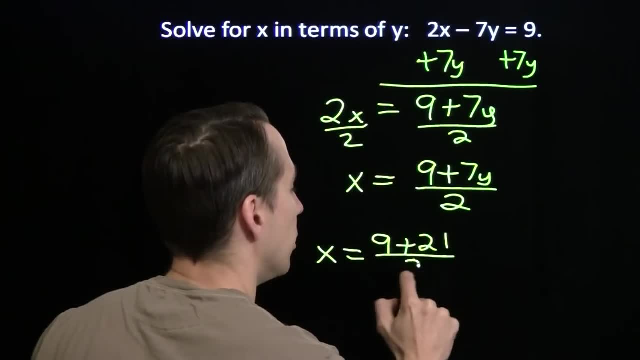 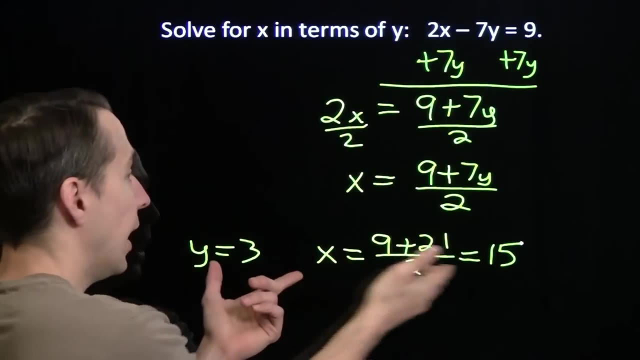 Suppose we decide y equals 3. Put that in here. We'll get x equals 9 plus 3 times 7 is 21, divided by 2.. 9 plus 21 is 30. Divide that by 2. You get 15.. Now let's test x. 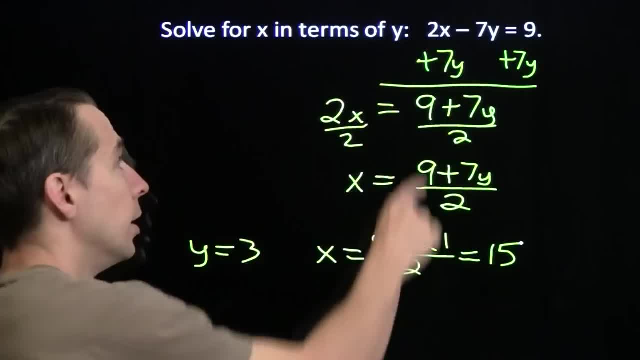 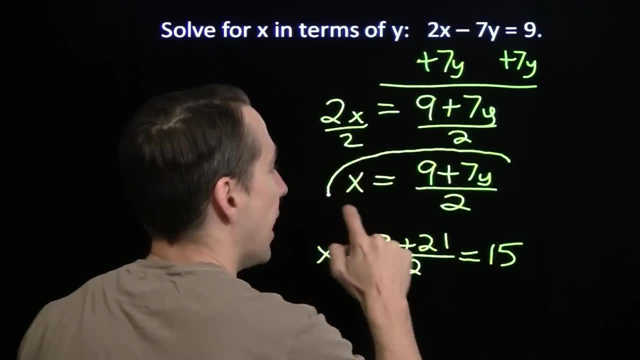 equals 15.. Put that up here: 2 times 15 is 30.. 7 times 3 is 21.. 30 minus 21 is 9.. It works. This is x, This is y, This is 2.. 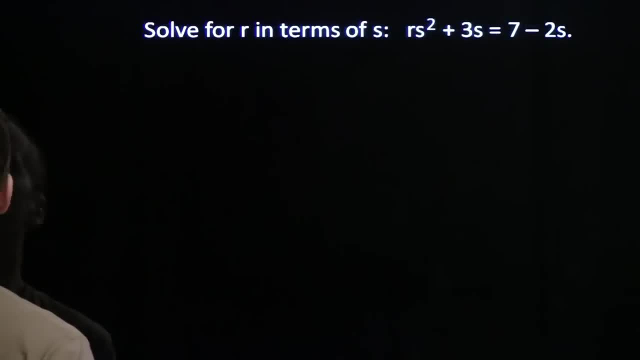 This is x, This is 2.. This is y In terms of y. Now let's try a slightly more complicated one here. We're going to solve for r in terms of s. Now let's look back here at what we did before. Our first step was to isolate. isolate the 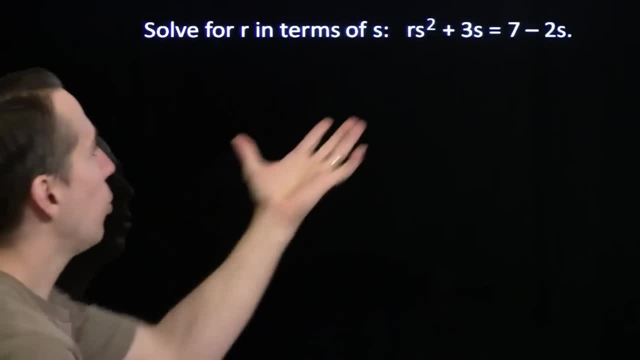 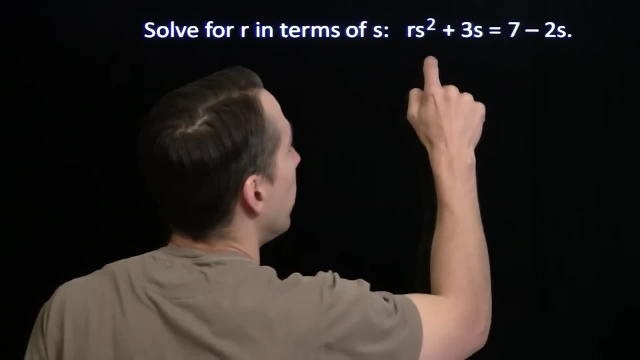 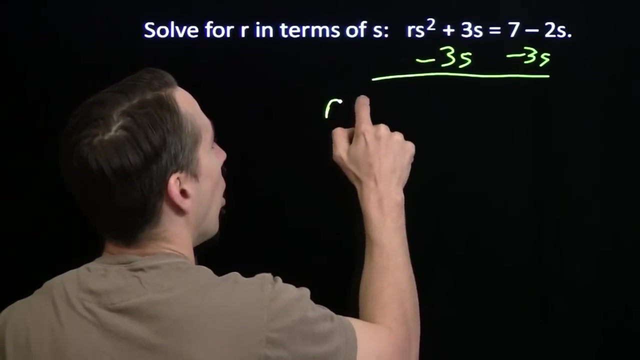 part of the equation that has x in it. So that's what we'll do here as well. Our first step will be isolate the part, the term that has the r, And we'll do that by subtracting 3s from both sides and we'll have R S squared equals 7 minus 2s minus 3s. 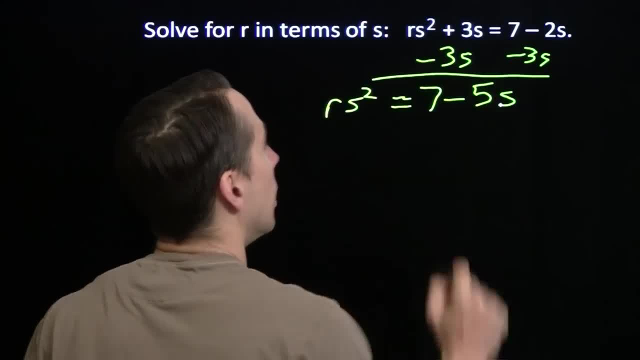 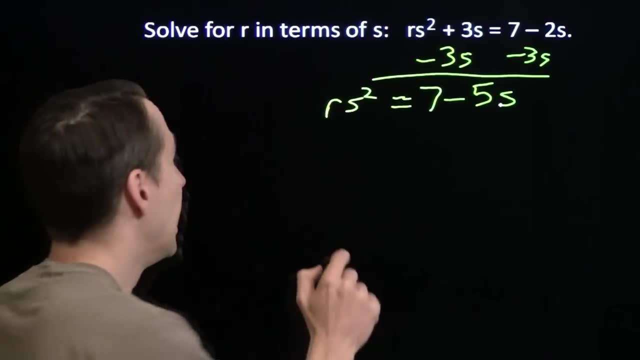 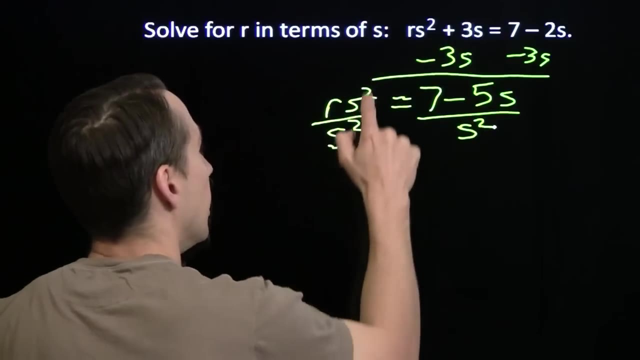 that's minus 5s. and then we need to isolate the R. well, we don't have a constant, a coefficient here that's multiplied by R, but we do have an S? squared and we can take care of that by dividing both sides by S squared. these: 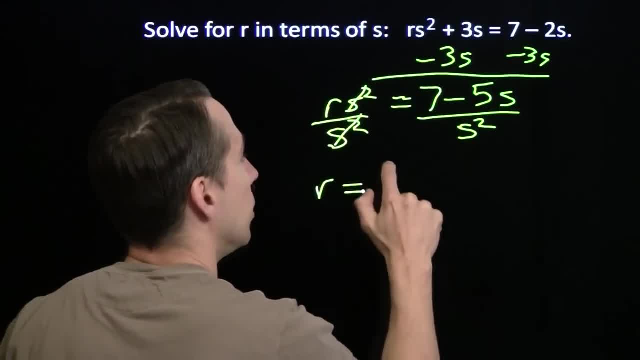 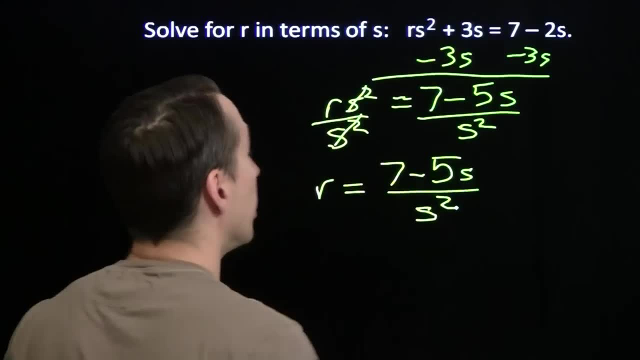 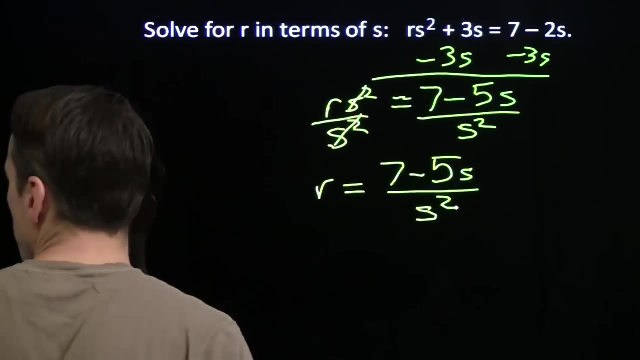 two S squared cancel and we're left with R equals 7 minus 5s all over S squared and once again we solve for R in terms of S. same thing we've been doing all along: we're isolating the variable. let's try one more. make sure we have this down. 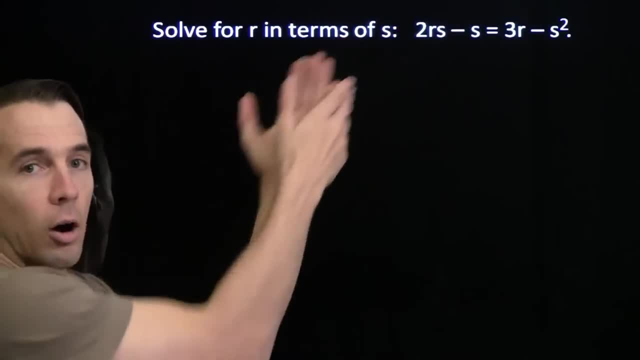 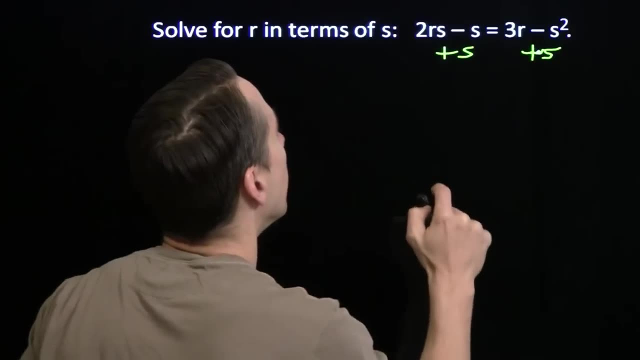 solve for R in terms of S. again, we're trying to get R all by itself. well, we'll start off the same way we did before. we'll just add the S to both sides and we'll get 2 R S, because the minus S and the plus S will cancel. 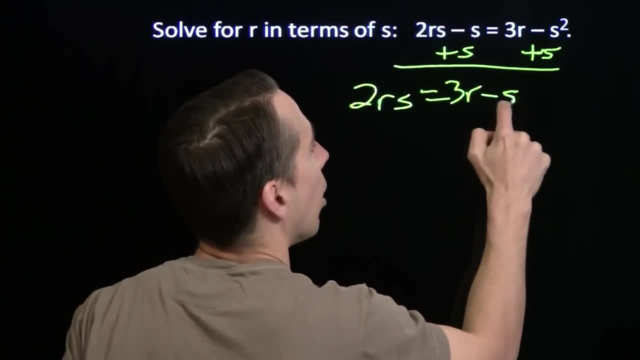 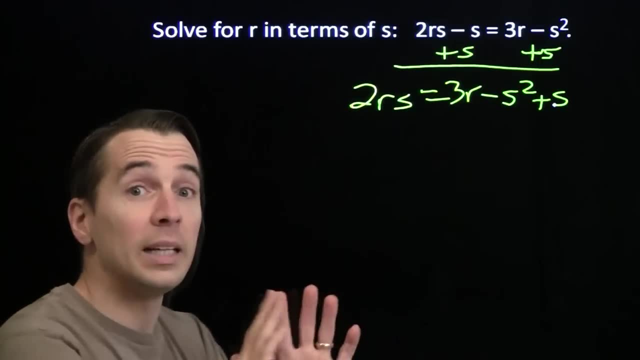 equals. we have a bunch of terms over here now: 3 R minus S, squared plus S. alright, so now we need to isolate the R. we need to get the R all by itself, so we have to divide by the 2 and by the S, because we want to cancel both of those. 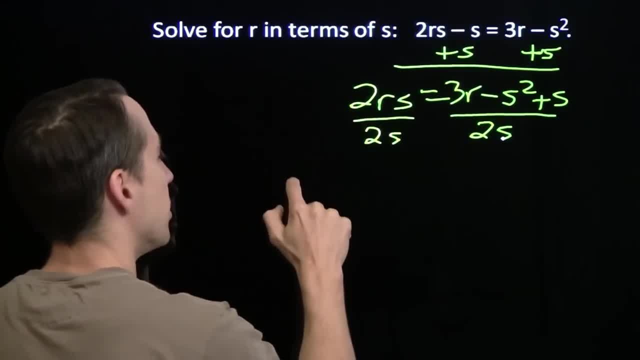 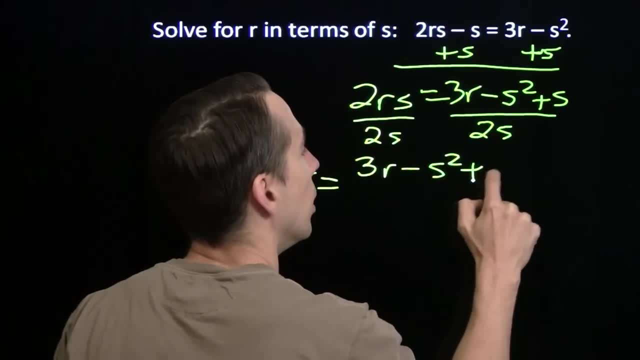 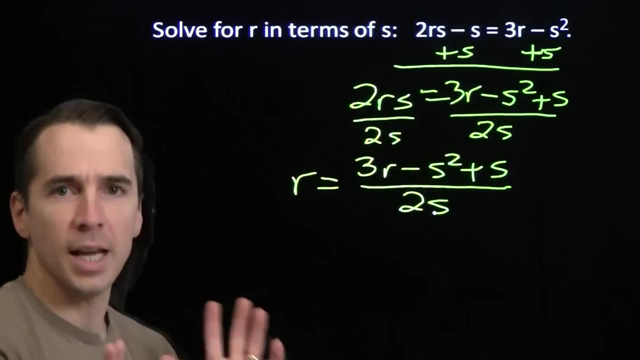 out and over here. we'll divide by the 2 and by the S and we'll be left with R equals 3 R, minus S. squared plus S, all over 2 S. alright, we should test this out. test this out. we tested out the same way we. 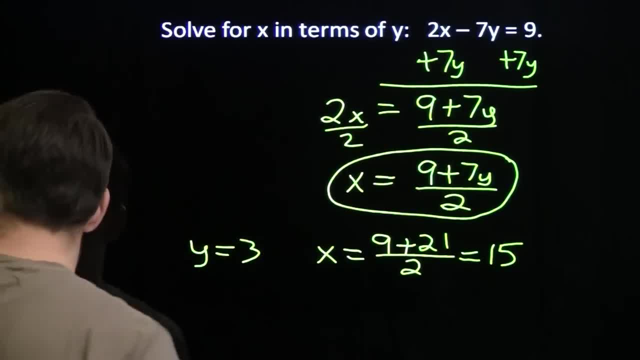 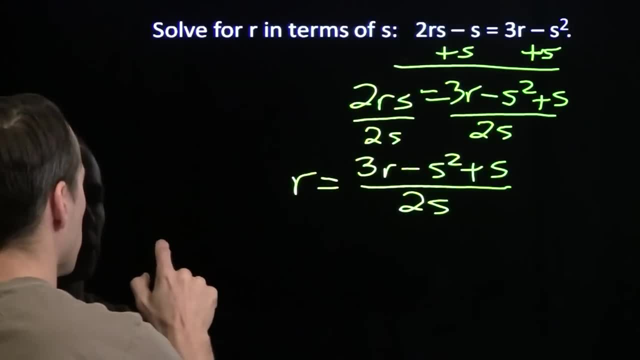 tested back here. we chose a value for Y, stuck it in, got X. we'll do the same thing here. just pick a value for S, put it in here, get R. see if our equation works alright. put in S equals 1 and we have R equals 3. 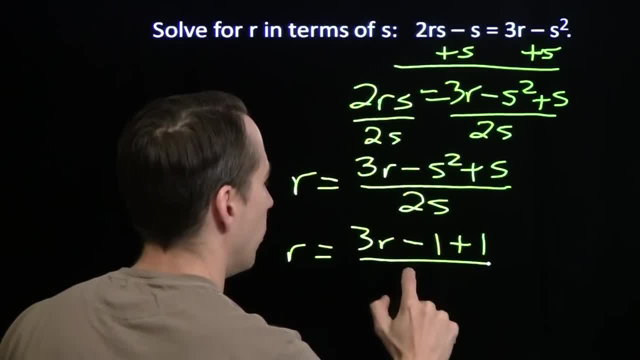 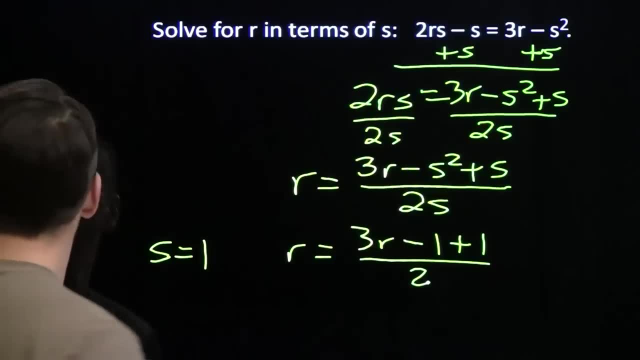 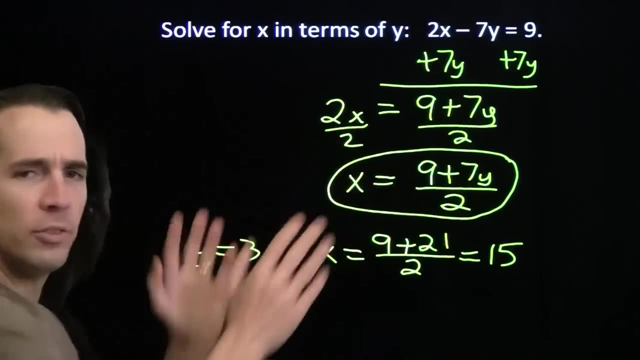 8r minus 1 plus 1 all over. wait a second. there are r's on both sides At the end. I'm supposed to have a nice little formula. I throw value for y in here. x comes out every time. 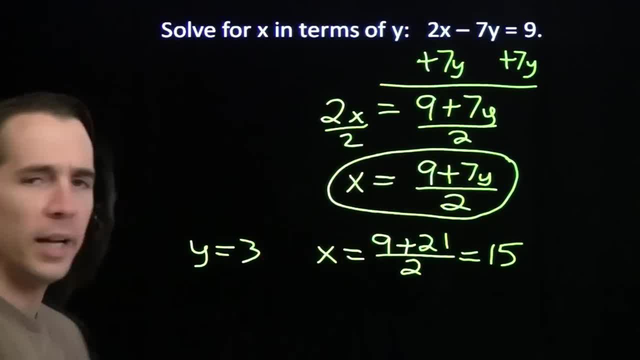 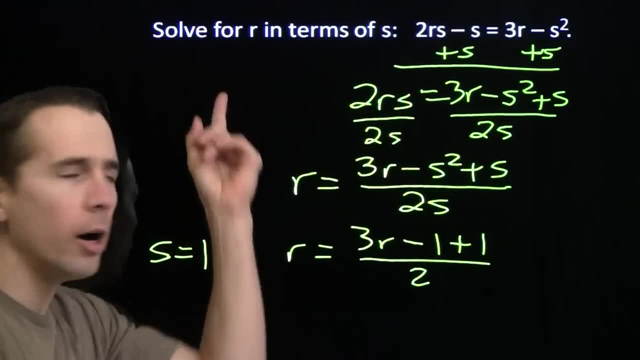 I don't have to do any solving an equation or anything. Once I have a value y, it's just arithmetic Here. I've got r's on both sides. I haven't solved for r. Ah, there are r's on both sides. 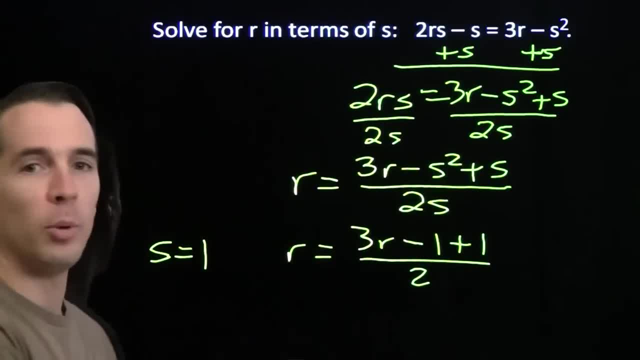 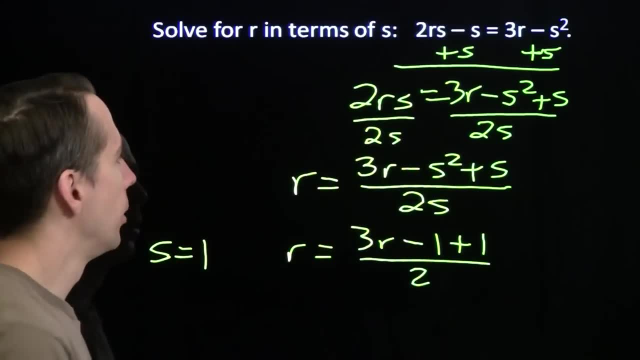 r is supposed to be alone. We're supposed to isolate the variable. That's what it means to solve for r. We have r equals stuff. that's not r, That's stuff that is r. Ah, what do we do? All right, you know what I do when I get puzzled, right? 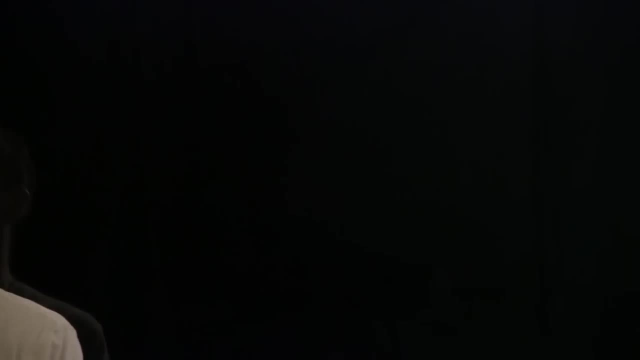 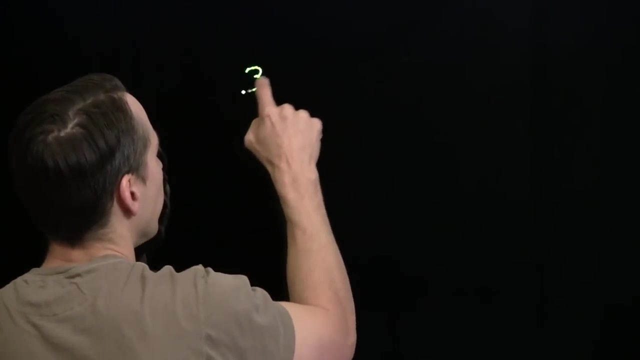 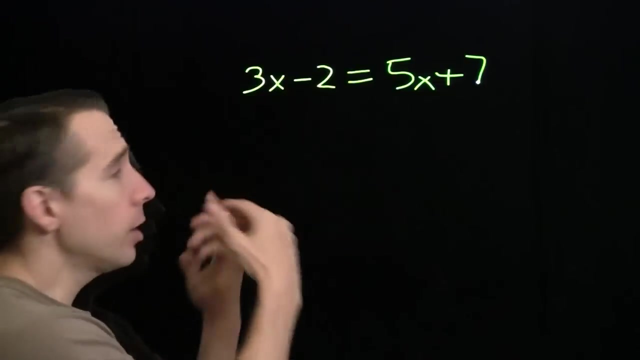 I think of a simpler problem that's similar to what I'm trying to do Now. the problem, the difficulty in that last problem, was that there's r's on both sides. If I had an equation, it was something like this: My first step is get all the variables over here on the one side, or all the variables. 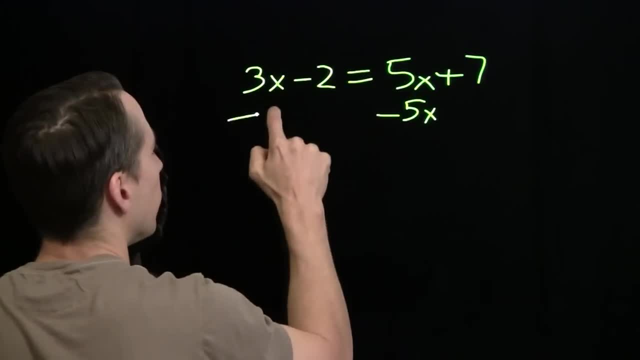 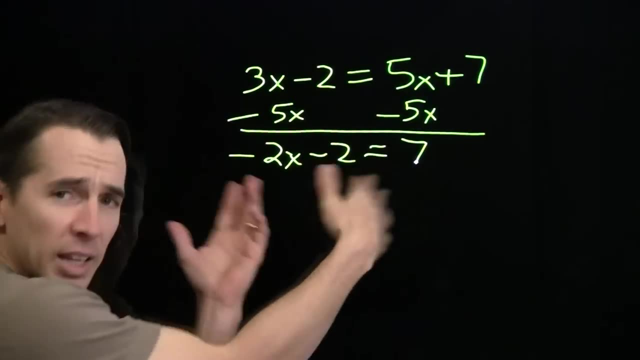 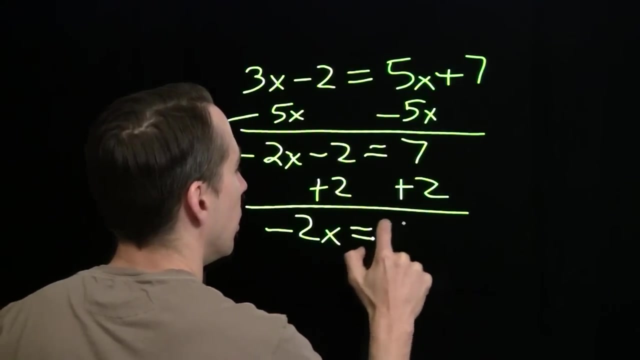 over on that side. It doesn't matter which, but if I subtract 5x from both sides, then I'll have minus 2x. minus 2 equals 7.. Then I can add 2 to both sides and I'll have minus 2x equals 9.. 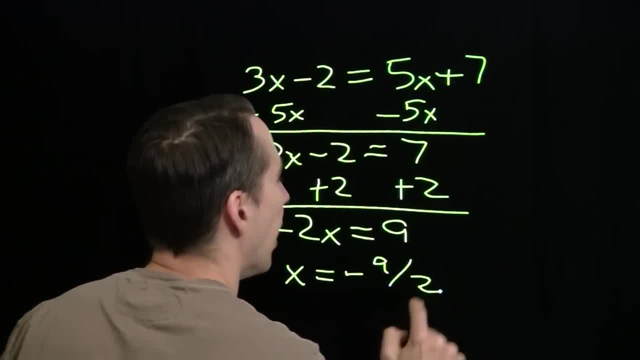 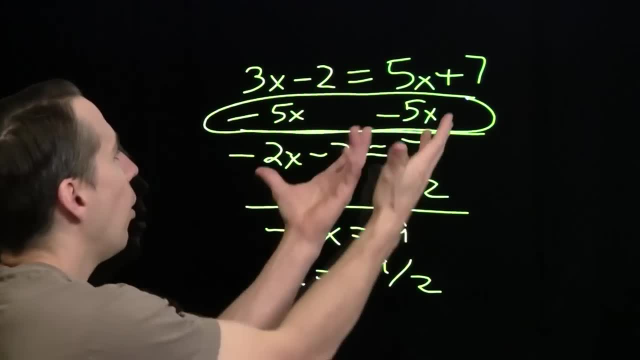 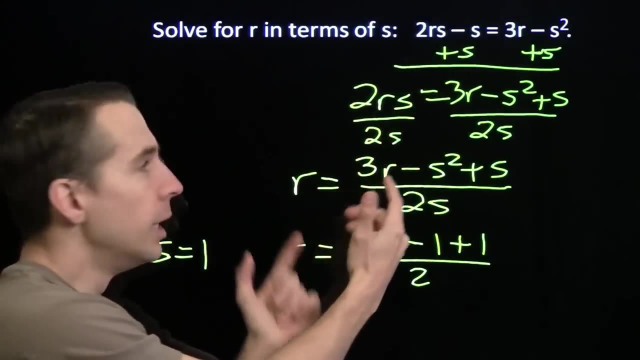 Divide both sides by negative 2.. I'll get: x is negative halves, Negative 9 halves. But my key first step here was this one: right here I got all the terms with x on the one side of the equation. That's what I needed to do here. 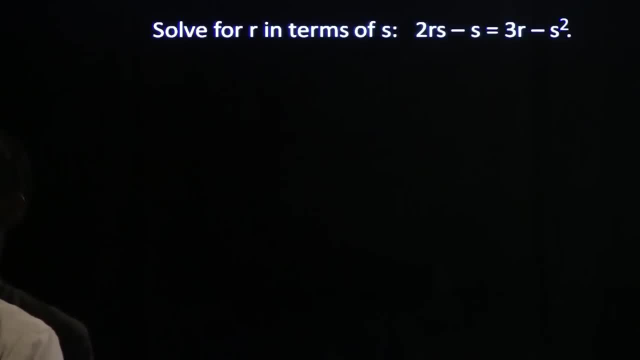 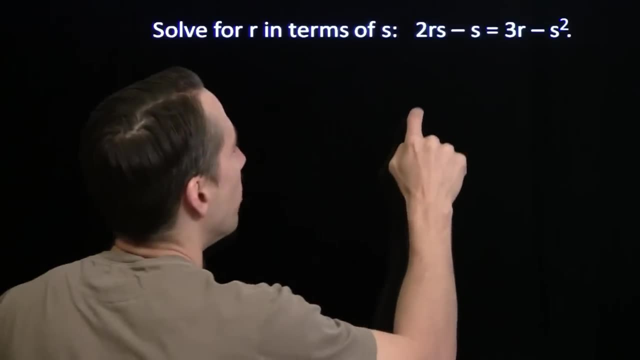 Get all the terms with r on one side of the equation. So let's start over and pretend that other thing. just forget it didn't ever happen, Never happened. I don't remember a thing. So our first step here: Let me now know what we have to do. 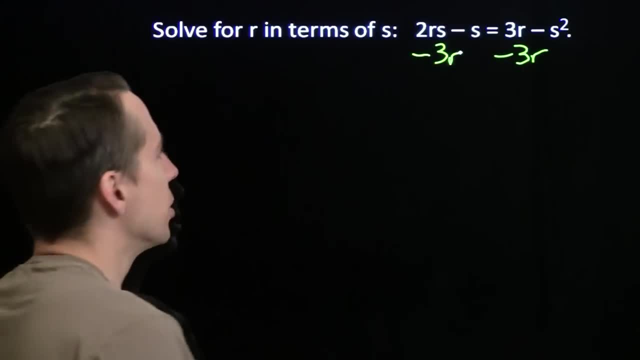 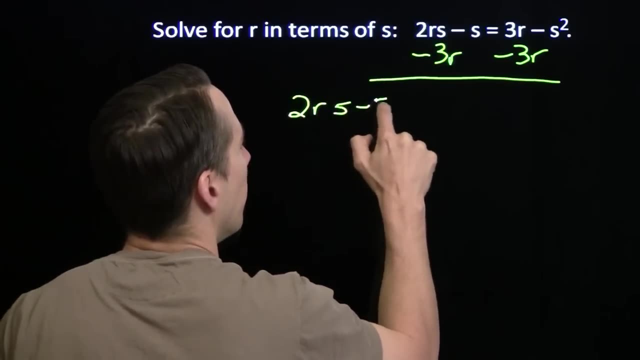 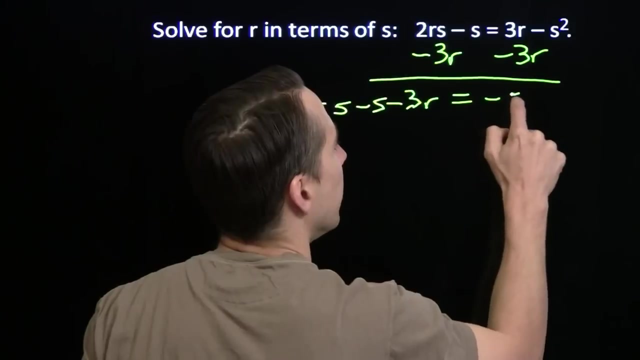 We're going to get all the r's on one side of the equation, Subtract 3r from both sides, and I'll have my 2rs, minus s, minus 3r, The 3r and the minus 3r. they cancel out and then I have minus s squared. 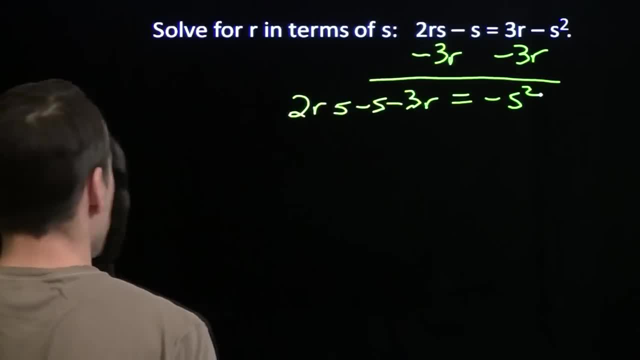 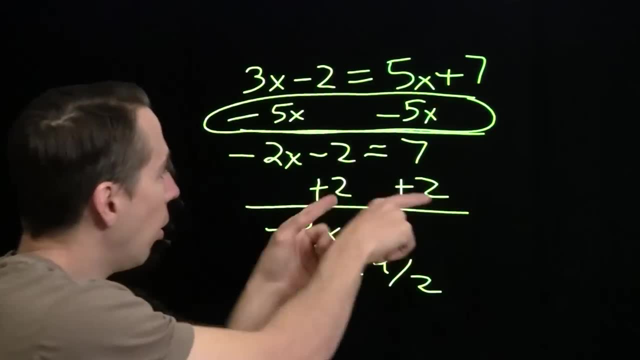 Now what? Well, I'll look back at my example, my simpler example, and maybe that'll help me. I also had minus s squared on one side. Oh yeah, that's right, I get all that not-x stuff over onto the other side of the equation. 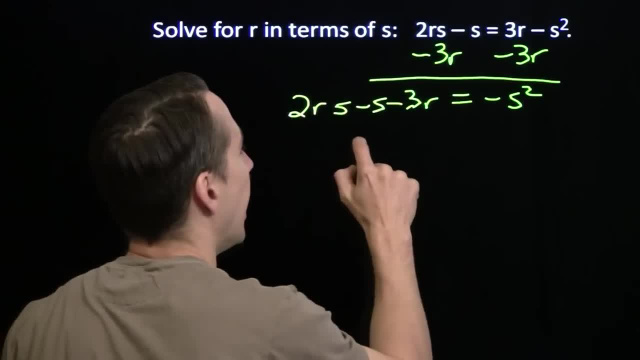 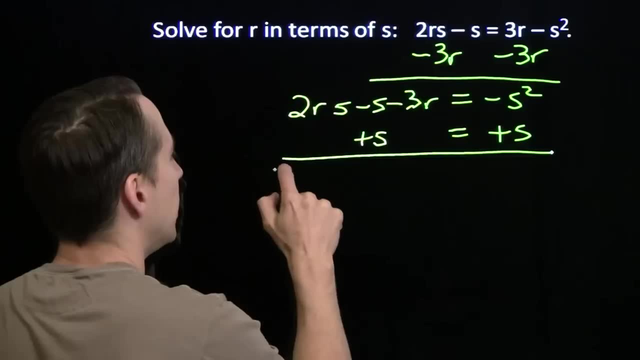 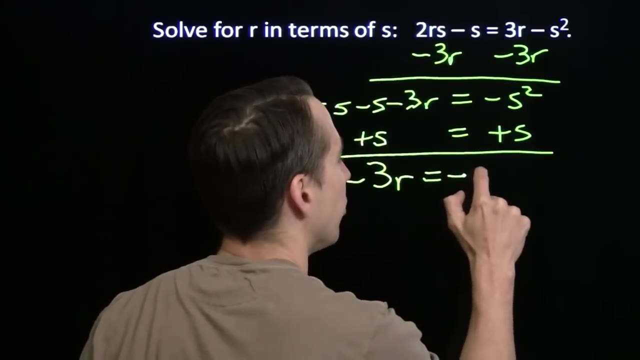 So we're going to take all the not-r stuff and push it over there. We're going to add s to both sides. So what's left over here will be 2rs minus 3r, and over here we'll have our minus s. 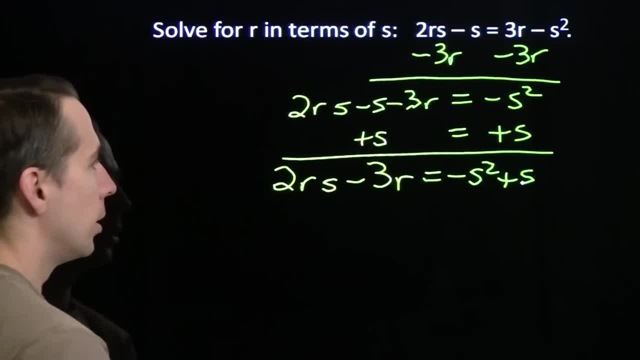 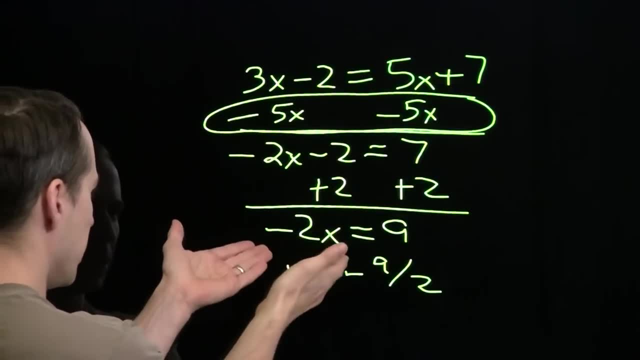 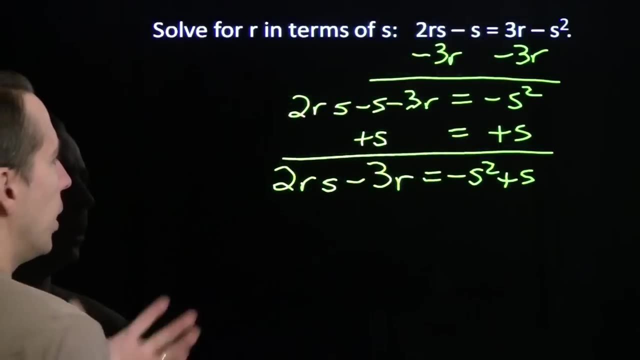 squared plus s, Adding s to both sides. Good, What more? Okay. Yeah, Now what? Okay over here, what we do? we have minus 2x equals. we divide it by negative 2, we divide it by the thing that's multiplied by the x. but over here we've got two things. 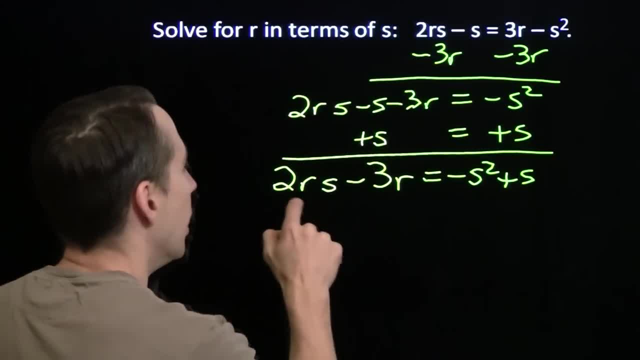 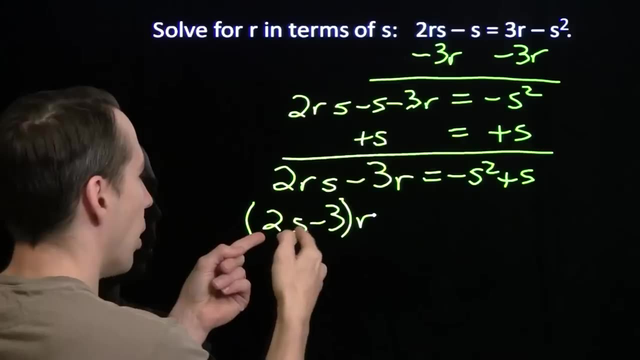 We can factor out the r and write this as r times. something Can factor the r out of this. need to grab my pen. factor the r out and we have 2s minus 3 times r. We can check that. multiply it back out: 2rs minus 3r. that all works just fine. 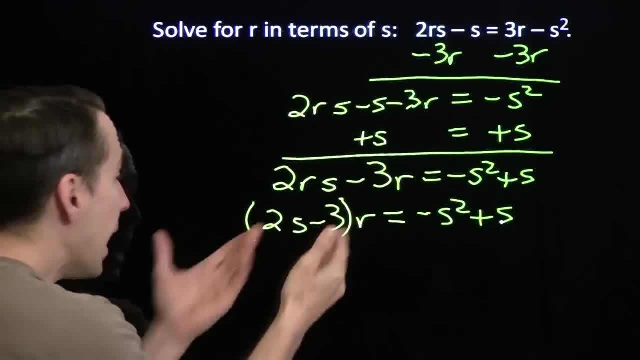 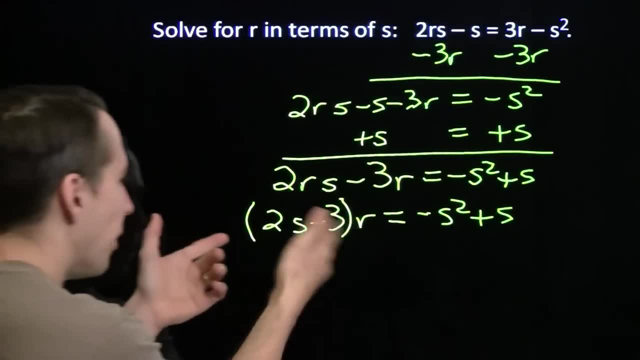 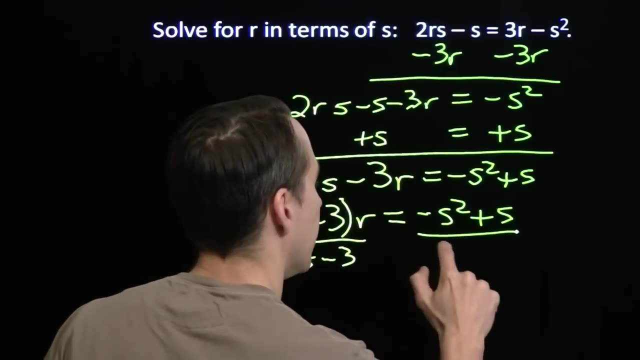 Alright, there we go. Now, if I look back here, we divided by negative 2. to get from here down to here Here, all we have to do is divide by the thing that's multiplied by r, dividing by 2s minus 3.. 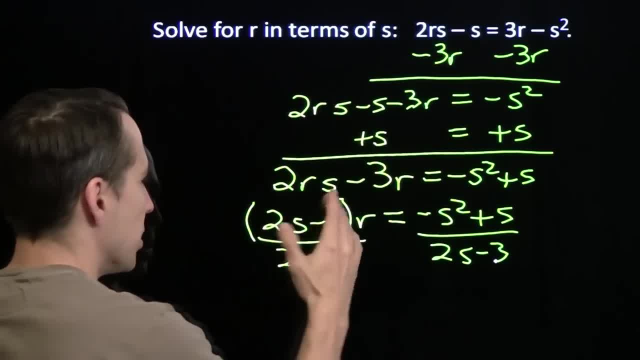 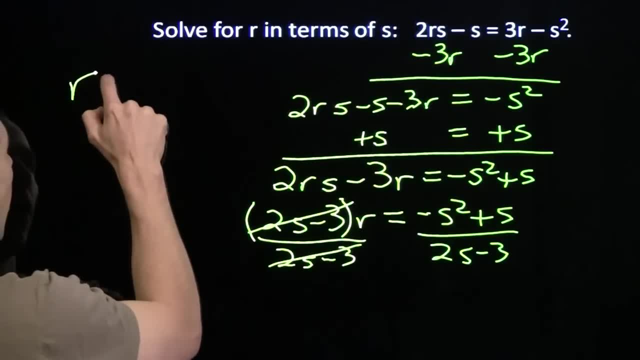 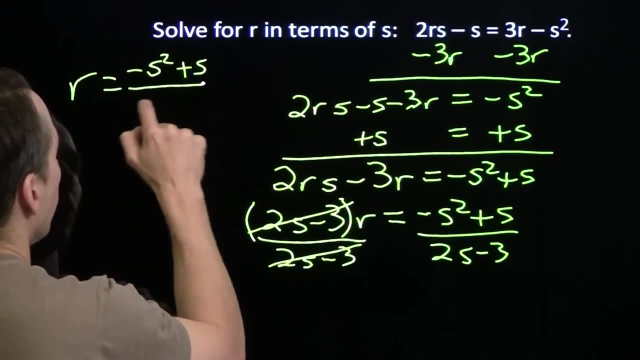 These are going to cancel, because this is just r times 2s minus 3 over 2s minus 3.. That is just 1.. So these cancel and we're left with r equals minus s, squared plus s, all over 2s minus 3.. 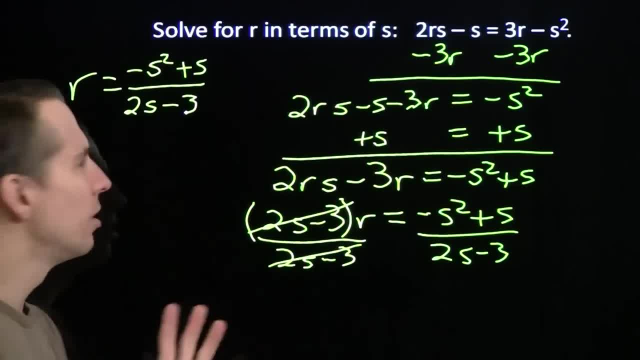 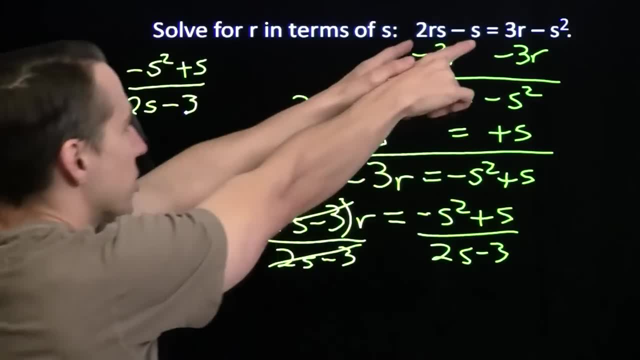 You know I want to test this. I'm going to test this a couple times. I'm going to stick a value of s in, get a value of r And make sure that that r and s works over here, because there's a lot of complicated.